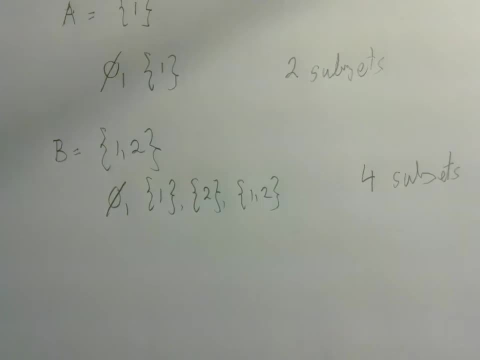 it will become more and more important that we're systematic. So the way we're going to be systematic is we're going to break down the listing by the number of elements in the subset. So let us work on a three-element set C that has one, two and three in it. 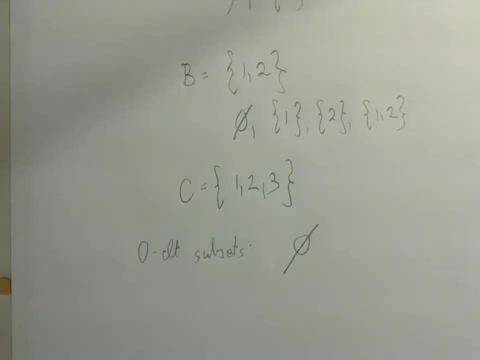 All right, so we have the zero-element subsets. That is just the one, the empty set For one-element subsets. well, we can have just one in the set or just two or just three, So there are three one-element subsets. 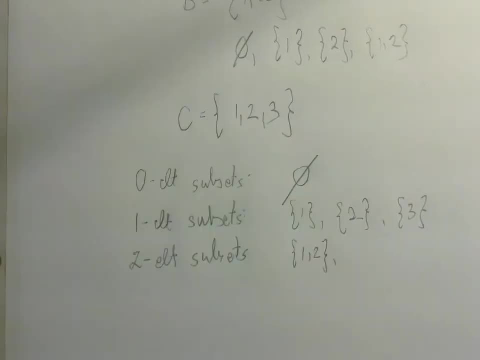 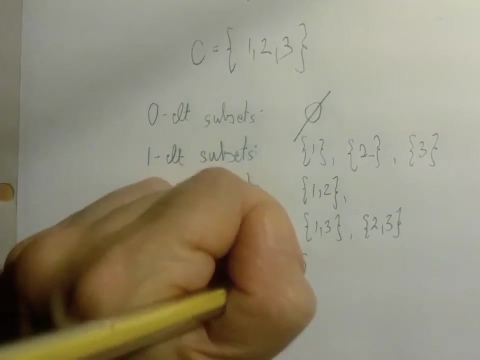 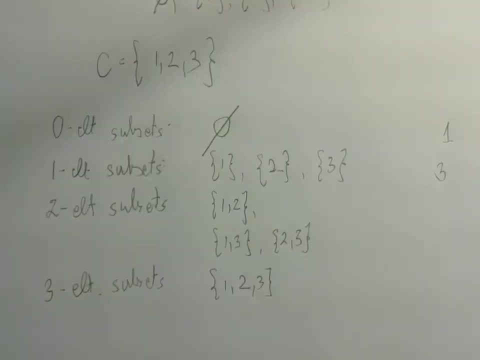 For two-element subsets there is one, two, one three and two, three And finally for three-element subsets, well, there is just the set itself. So we had one zero-element subset, three one-element subsets, three two-element subsets and one three-element subset. 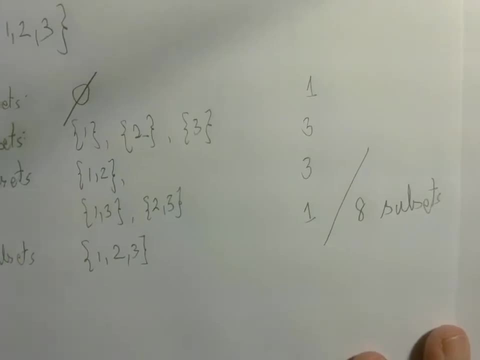 So altogether eight subsets. Let's see the subsets of a four-element set D, containing the numbers one, two, three and four. For zero-element subsets there is just the one, the empty set. For one-element subsets. well, there is four ways we can pick one. 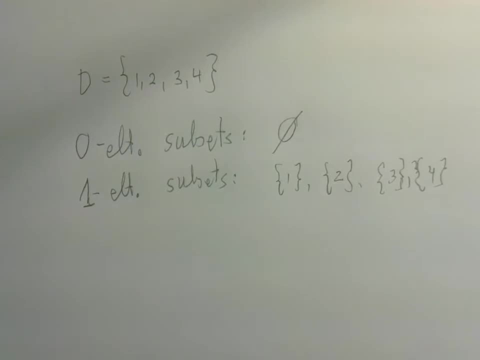 So we're not exactly surprised that there are four such subsets. Now it's getting a little stickier. Let's see the two-element subsets. So there is one, two, one, three, one, four. So we're done with the two-element subsets with one in them. 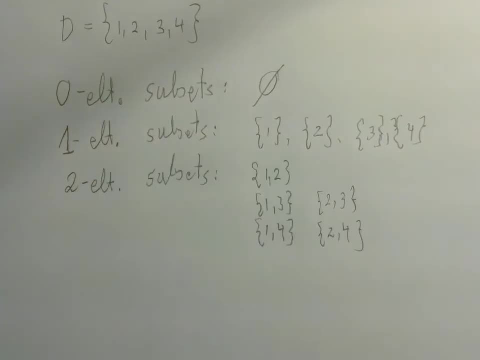 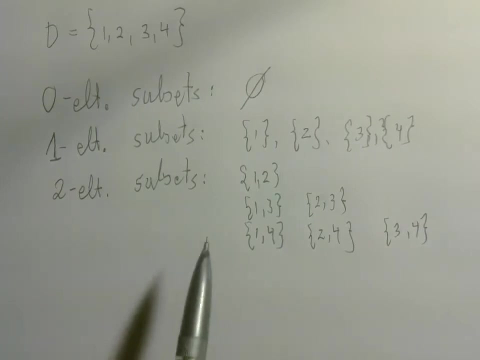 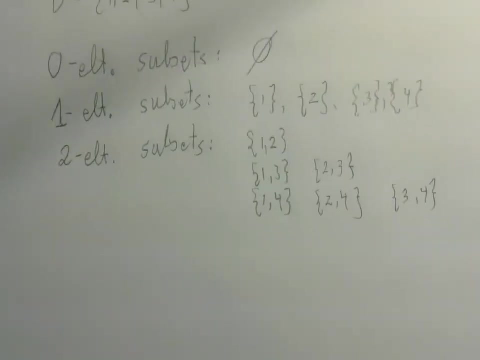 Let's roll up to two, two, three, two, four and three, four. Now notice that, being organized or being systematic, one tool in it is the visual arrangement. See, I didn't write just one line. We have this nice triangular shape. if we use the spatial arrangement as a tool of organizing, 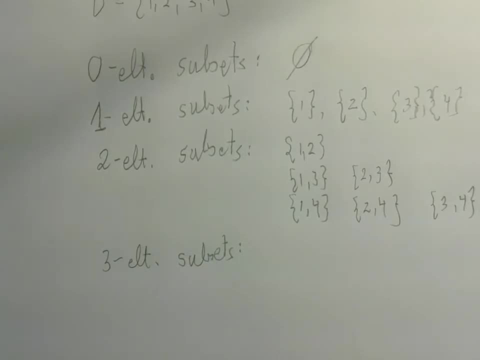 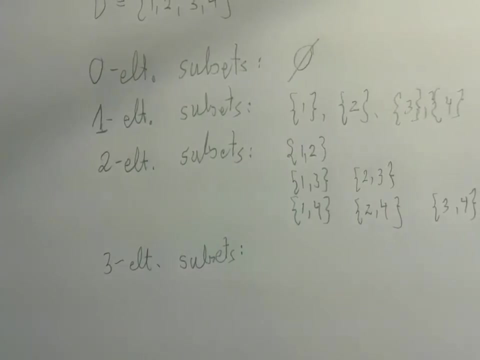 Now for the three-element subsets. I propose a new trick, And that is, instead of building up the subset from scratch, because three is almost four, why don't we just start with the entire set and just pick one thing that we throw out from the set? 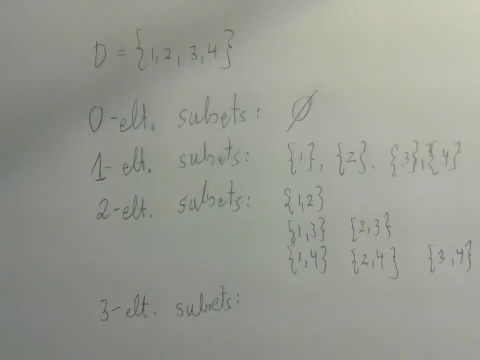 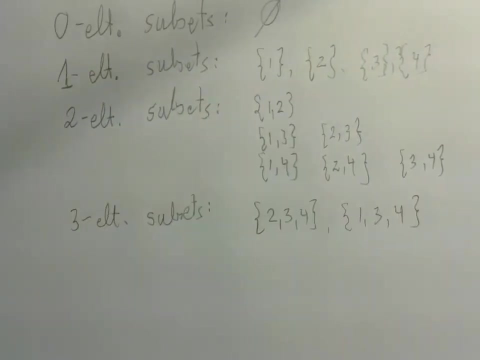 So we could start with the set one, two, three, four and kick out one, Then we get two, three, four. Or we can kick out two, then we get the set one, three, four. Or we can kick out three, then we get one, two, four. 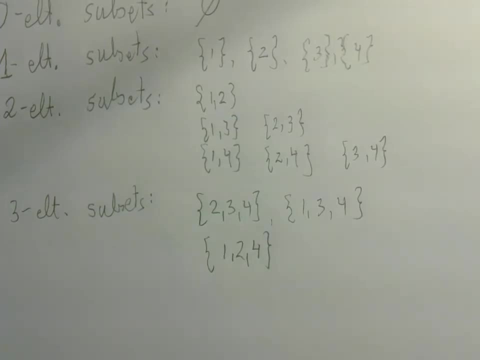 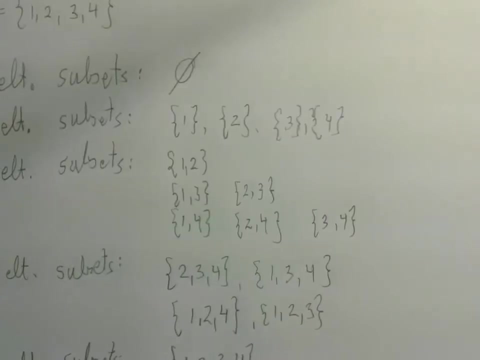 And finally, when we kick out four, we get one, two, three And for four-element subsets there is just one: the set itself. So let's see, For zero-element subsets, we had one, For one-element subsets, we had four. 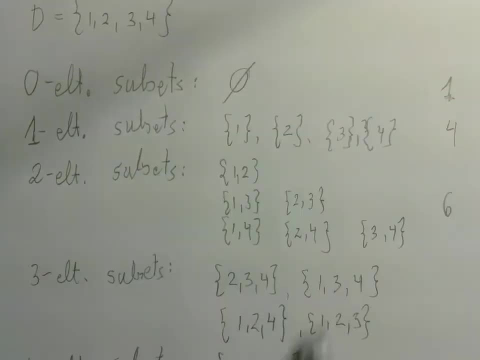 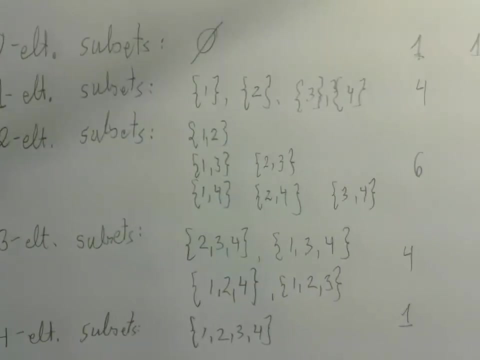 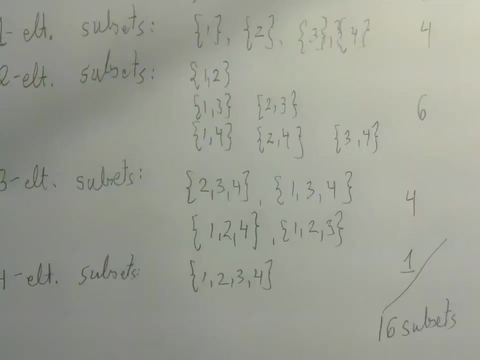 Two-element subsets, we had six. Three-element subsets, we had four And just one four-element subset in a four-element set. So all together we have sixteen sets. There is a pattern here, right? If the set had one element, we had two subsets. 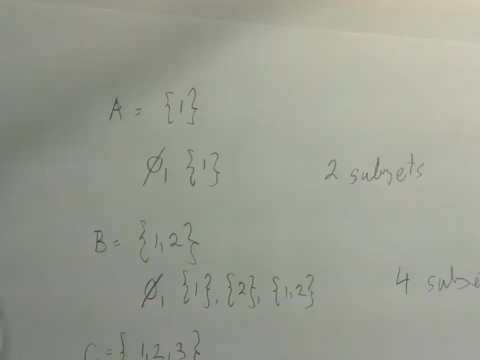 If the set had one element, we had two subsets. If the set had two elements, we had four subsets. If the set see one, two, three had three elements, we had eight subsets And we had to work for it a little bit. 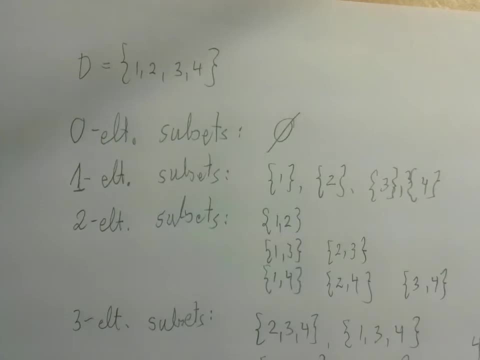 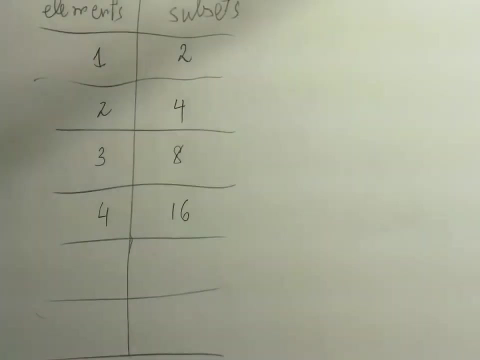 But if the set had four elements, like one, two, three, four, then the number of subsets was sixteen. Do we predict that if we move up to a five-element set will we get thirty-two, Even if you're already sure it's not a bad idea to list four subsets? 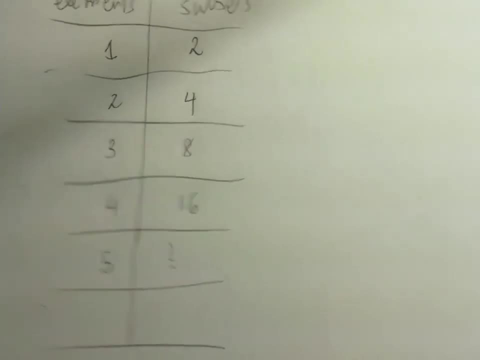 Let's list this one more and then I'll promise we'll stop. You can fast-forward. So let's say we're listing the subsets of the five-element set E containing one, two, three, four and five. So for zero-element subsets there is just one, the empty set, right? 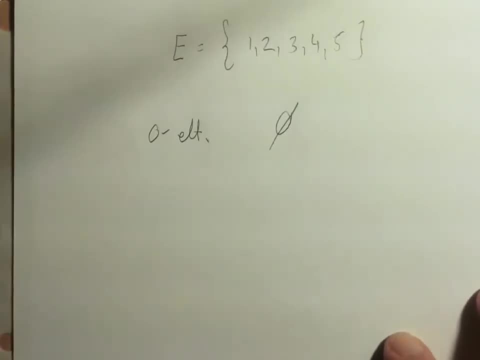 For one-element subsets. well, we can predict five of them. right, It's either one alone or two or three, or four or five alone. For the two-element subsets, let's see: There is one-two, one-three, one-four, one-five. 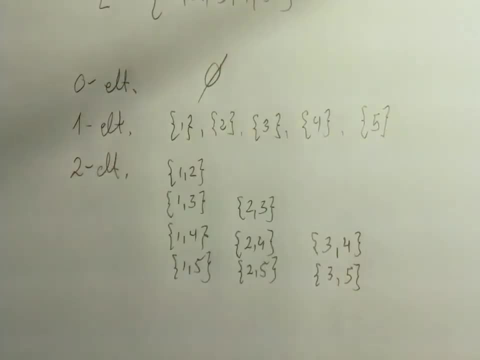 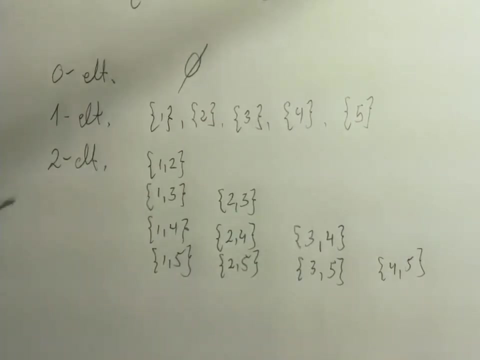 two-three, two-four, two-five, three-four, three-five and four-five. We get this nice triangular arrangement, And the reason we're doing this listing is these are becoming interesting questions: How many four-element subsets in a ten-element set? 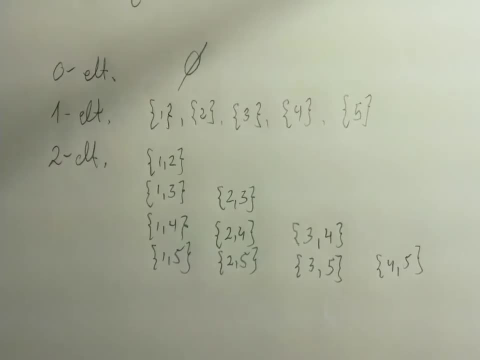 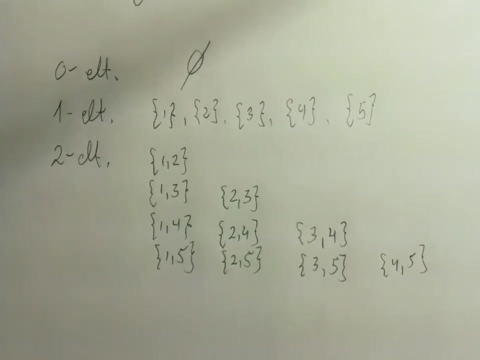 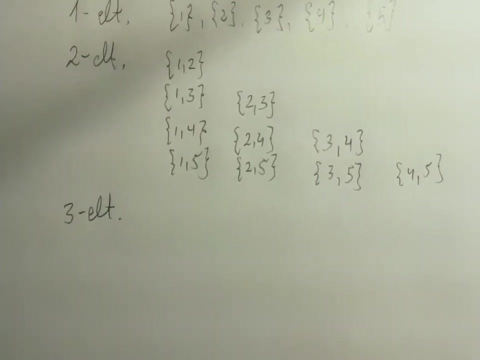 By the time we figure out the total number of subsets. this, broken down by the number of elements of the subset, becomes interesting and more difficult. So let's see the three-element subsets in a five-element set. That's going to be tricky, even with the spatial help. 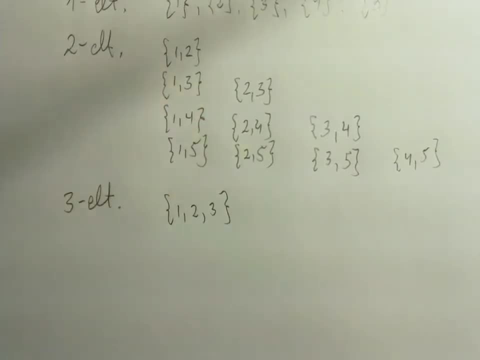 There is one, two, three. So, to be organized, we're going to fix one and two And run with it as far as we can. One-two-three, one-two-four and one-two-five. Let's roll up to one-three, one-three-four, one-three-five and one-four-five. 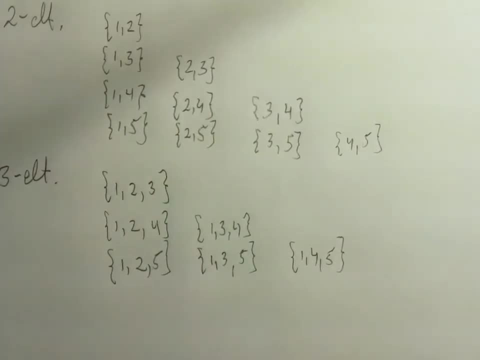 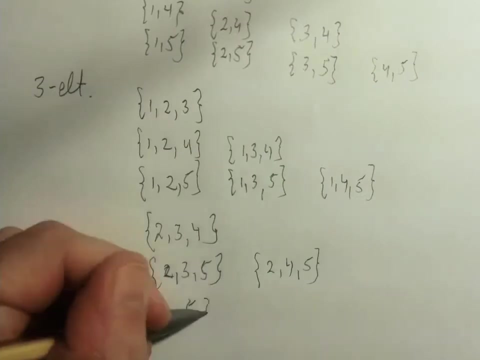 So these are just the ones that have one in them. Now let's roll up to two. So there is two-three-four, two-three-five, two-four-five and finally three-four-five. Okay, so now for the four-element subsets. 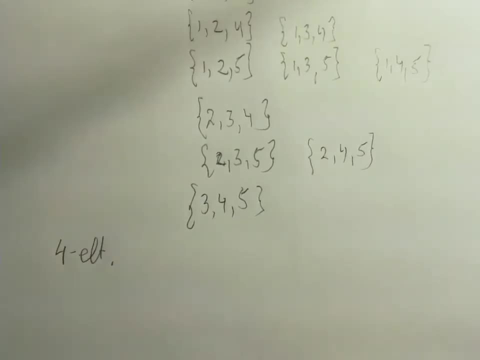 we're going to apply the same trick. So, instead of building up the set from scratch, we're just going to grab the entire five-element set and kick out just one element. So we can kick out one, then we get two-three-four-five. 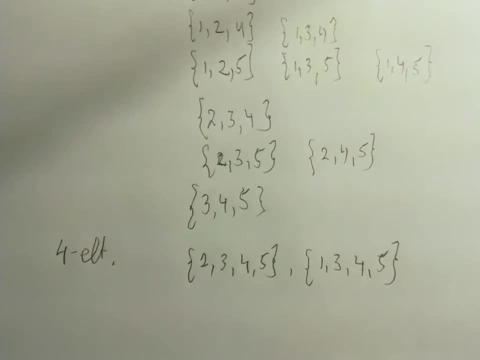 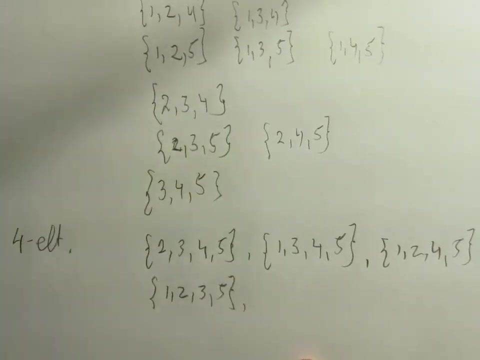 We can kick out two, then we get one-three-four-five. We can kick out three, then we get one-two-four-five. We can kick out four, then we get one-two-three-five. And finally, we can kick out five, and then we get one-two-three-four. 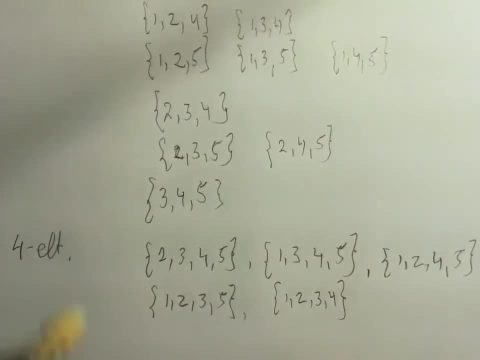 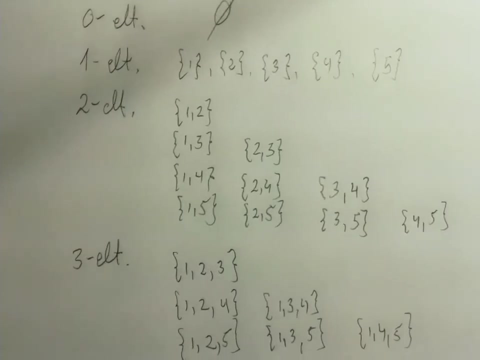 So notice right away that the number of four-element subsets is going to be the same as the number of one-element subsets, and with good reason, Because in a five-element set for a one-element subset we have to choose one out of the five. 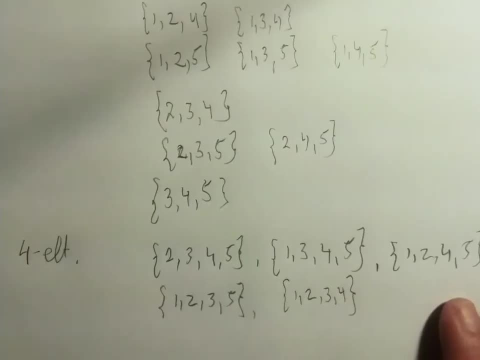 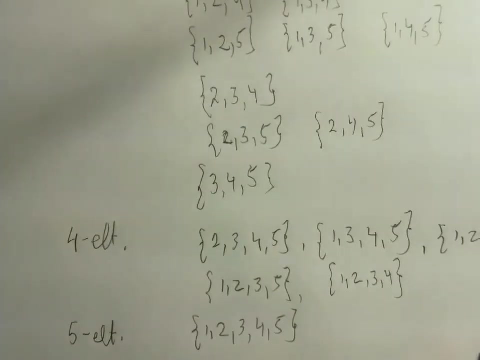 but so do we for the four-element subset. We just pick one element to kick out from the set, right? So there is some sort of symmetry going on here. Finally, for the five-element subsets, there is just one: the set itself. 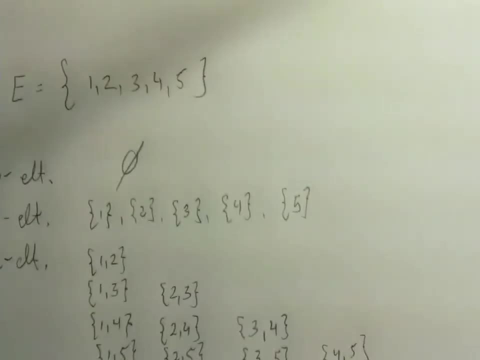 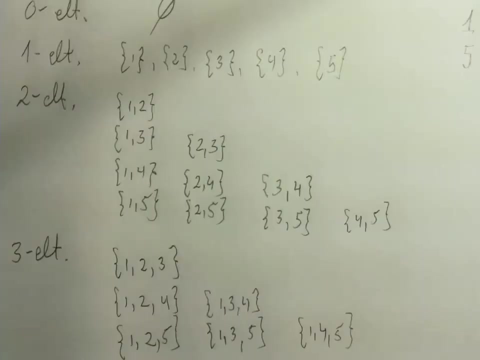 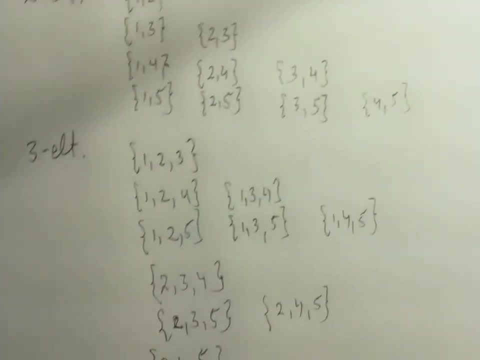 So now let's see how many subsets do we found? So the zero-element subsets, there was one. Four. For one-element subsets, we had five. For two-element subsets, we had four plus three plus two, That's ten. And probably the three-element subset was the trickiest. 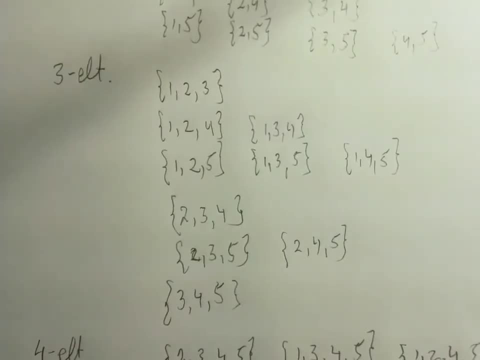 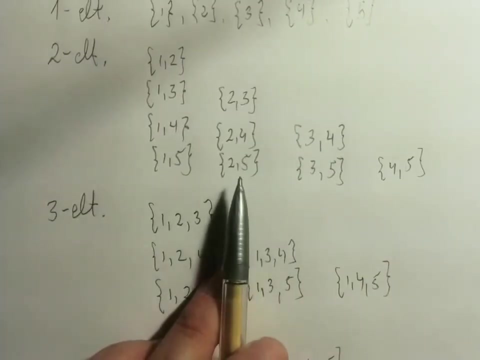 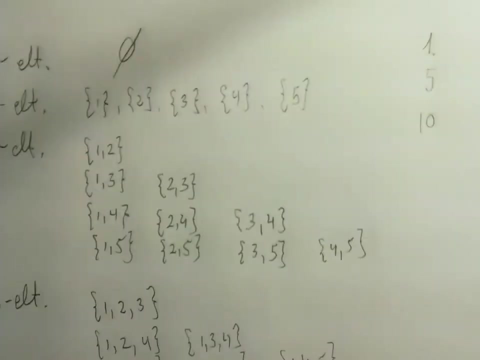 But now we could argue that we could have started with the set itself and just kicked out two. So selecting two elements to put in our set has to be the same number of ways possible as selecting two elements to kick out from our set. So we have ten of each. 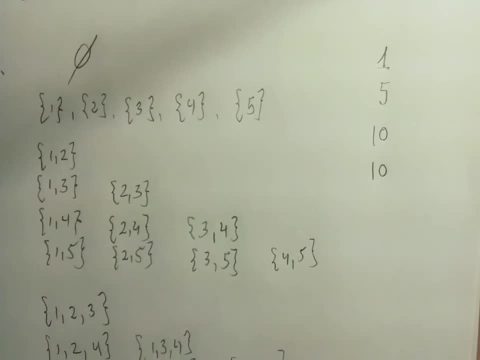 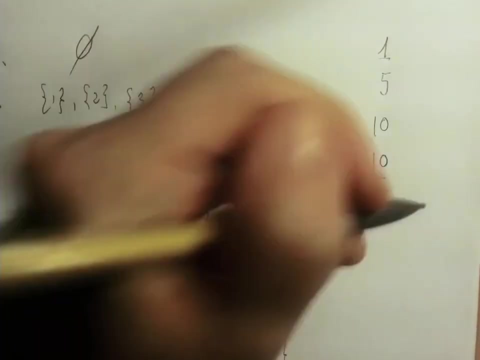 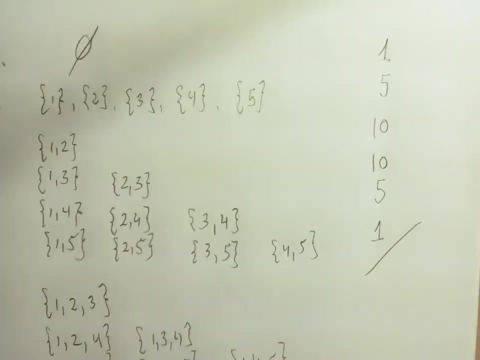 We have ten two-element subsets and we have ten three-element subsets of a five-element set, The four-element subsets. there were five, many And finally just one five-element subset, So we have 32.. So our suspicion was confirmed that if we move up to five, 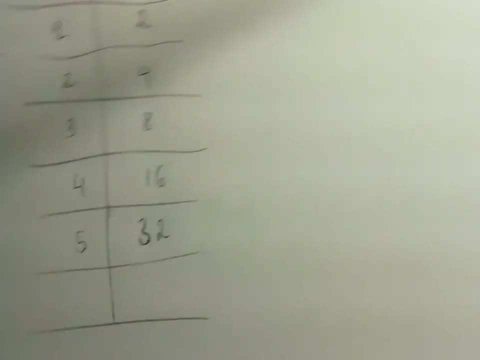 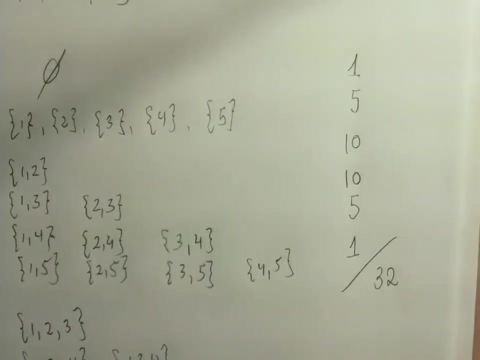 the number of subsets is indeed 32.. Will this keep? Will we get 64 next? But also we discovered- I promised you- that by the time we answer one question, we're going to have many others. There is some sort of a symmetry going on. 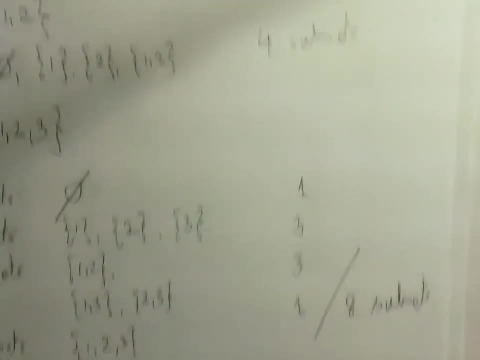 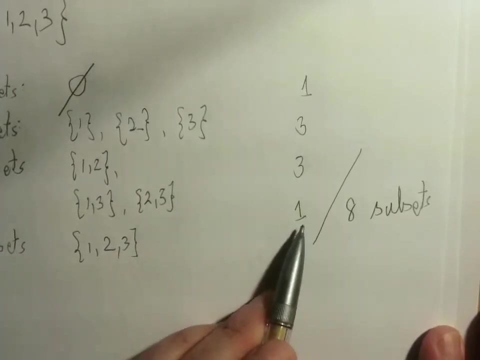 even if we go back. Let's look at the three-element subset. The zero-element subset is the same as the three-element subset Picking nothing- picking nothing to throw out The one-element subset and the two-element subset picking one number, or picking one number to kick out. 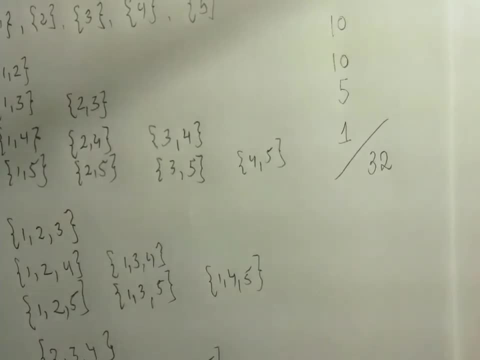 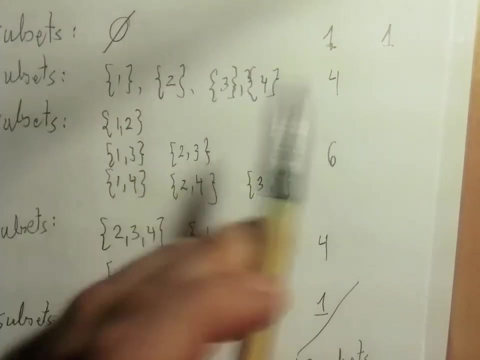 Now for a set. we have three elements, or we just did that, Four elements. there is the symmetry again: One, one, four, four, six. So the number of one-element subsets in a four-element set is the same as the number of three-element subsets. 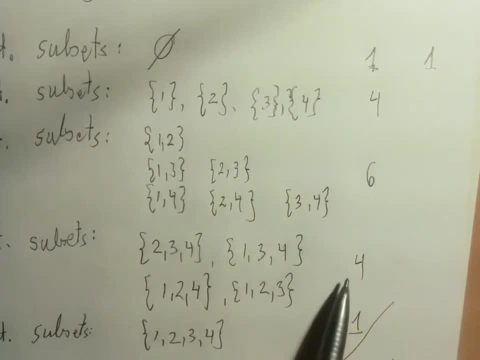 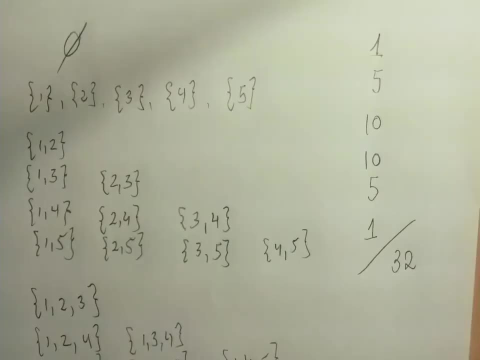 Because here we pick one to select into our set and here we pick one to kick out from our set. So there is this sort of outer symmetry that it looks like we have good reasons for that. Okay, The other new difficult question is: 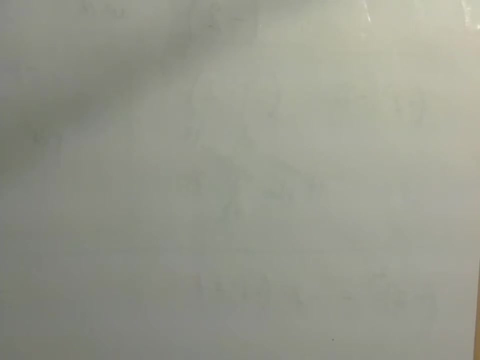 it looks like we're going to figure out how many subsets to a set, But what about this broken down, Like, for example, how many three-element subsets in a ten-element set? So this is a new question that we bumped into as we were trying to answer, as it turns out, an easier 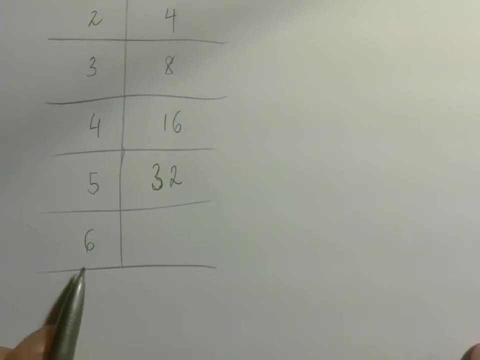 Now let's see how we could figure out what happens with six or seven or eight. Will this doubling thing persist Or will we lose it? We just figured out that if we have a set E- so we just figured out that if we have a five-element set. 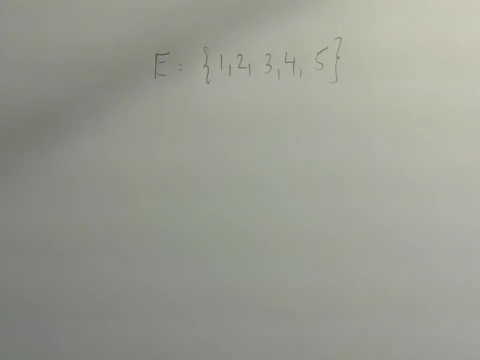 then there is 32 subsets right Now. let us imagine that we write them into one long column. So there was the empty set, there were the one-element subsets, there were the two-element subsets, and so on all the way till the set itself. 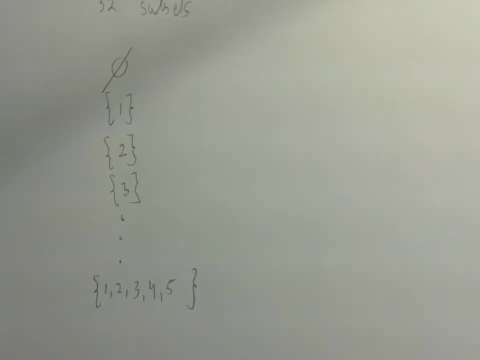 Okay, So here comes the trick. We're going to copy this entire column, So we're going to double it, And now we have the following: In each column, every single subset is different, And the same is true here. It's just that this is equal to this. 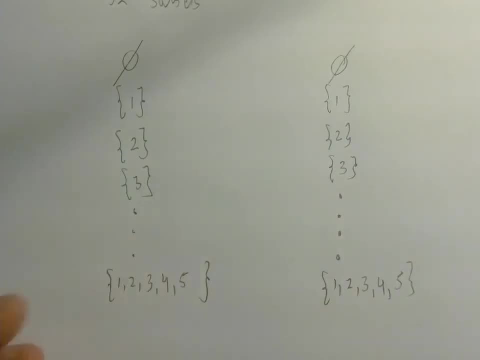 this is equal to this, and so on, But we're going to mess that up. So now, here is what we're going to do. Consider the set F, which we get by throwing in six into our old set, And now what we're going to do. 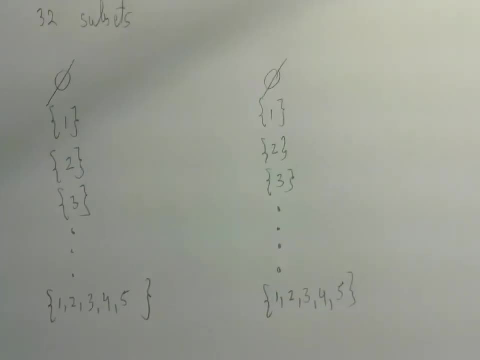 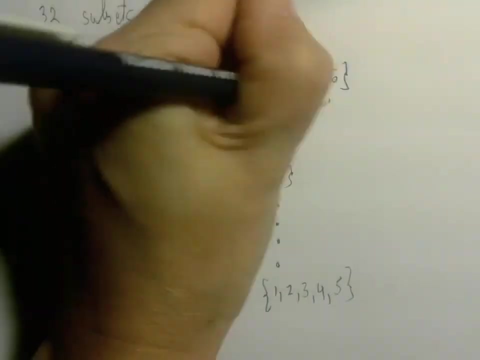 we're going to go into the second column and we're going to throw in six into every single set. So the empty set will become the set containing six, only The one-element set. one will become a two-element subset. one, six. This will become two six. 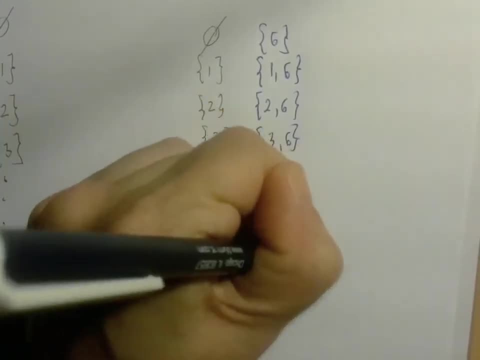 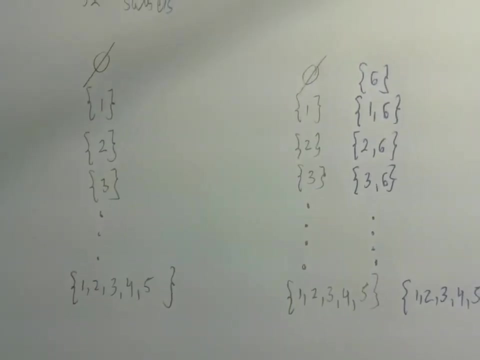 three, six and so on. The last one will become one, two, three, four, five, six, And now we have 64 subsets. right Now, remember that in each column all the subsets were different, And here they remain different in the second column. 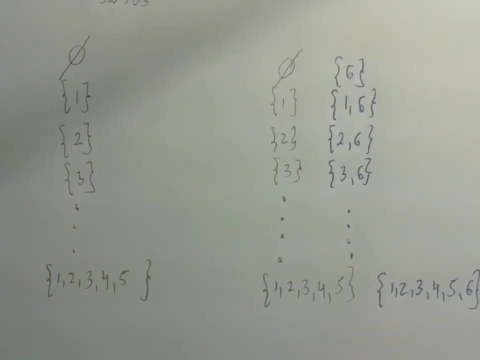 because we did the same thing to them. We just threw in the six And not one. set from the first column equals to any set in the second column, because the second column has subsets with six in them, The previous one doesn't. So we doubled up from 32 to 64 subsets. 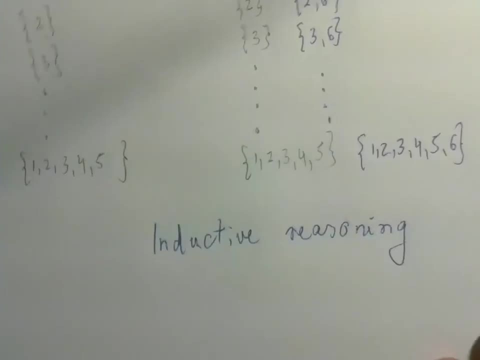 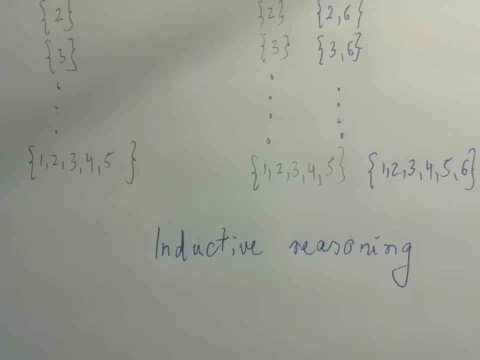 So this is what we call inductive reasoning, where we sort of build on our previous result to figure out the current one, And then we preserve that and we use that to figure out the next one. So we're building on our previous result. so a six element set has 64 subsets. 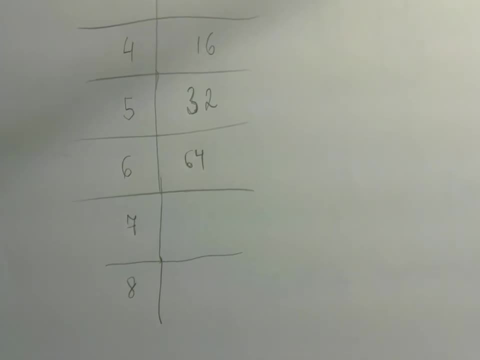 We line them up to a long, long column, We repeat that column And into the second column, into every set we throw in seven. That way we get 128 subsets And notice that it doesn't even just double. but it has a very nice pattern here. 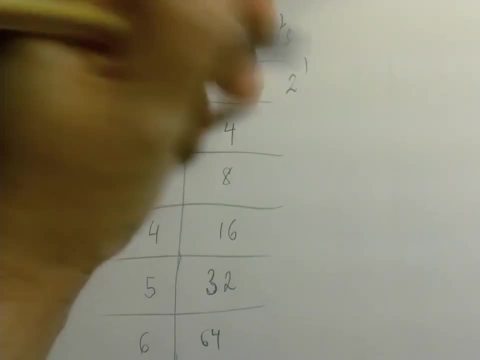 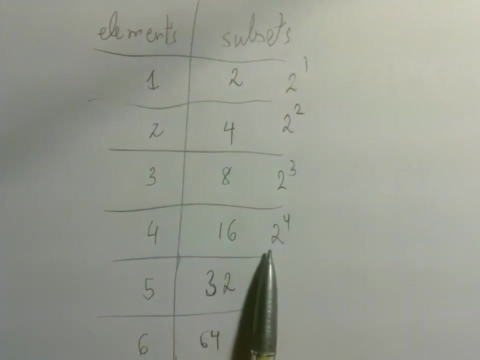 because two is two to the first power, Four is two to the second power, Eight is two to the third power. So it looks like the formula for the number of subsets is: take two and as exponent use the number of elements in the set. 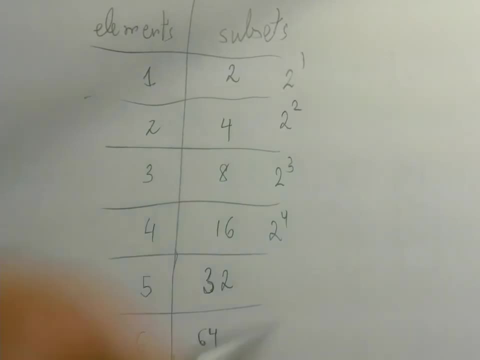 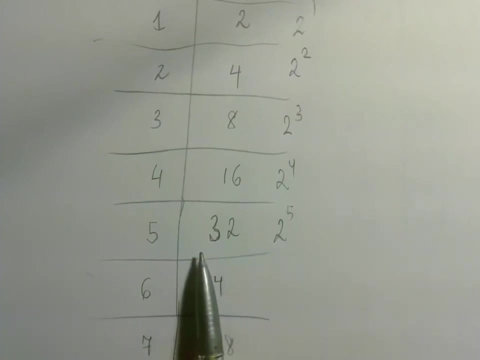 And that's how many subsets are there? Indeed, 32 is two to the fifth power. So a five element set has two to the fifth power, or 32 subsets. This is true. So this is our theory, that if we have a set with n elements in it, 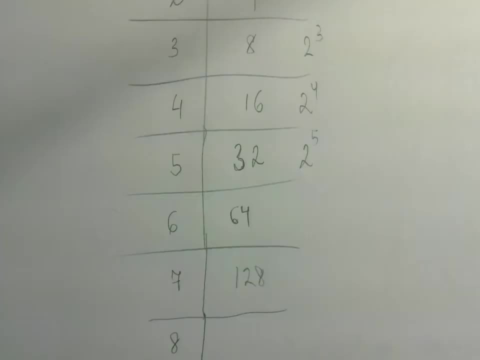 then the number of subsets is going to be two to the nth power. Now, as it turns out that we can list all the subsets and then put them into a set, That's going to turn out to be an important set, And because of the size of this list, 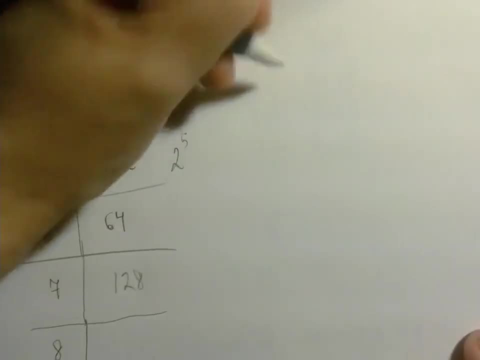 it's called a power set. I speculate because it's a two power. So the power set of a set is the set of all subsets to the set. I believe that if we start with systematic listing, we bump into this inductive way of figuring out the number of subsets. 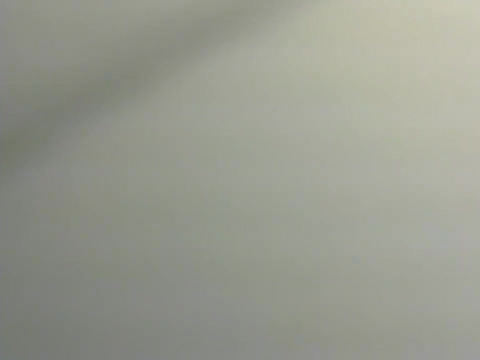 But now that we know the answer, there are easier, more intuitive combinatorial ways to argue for that. Let us consider the set one, two, three. Now, instead of listing all the sets, this is called constructive counting. Constructive counting is: 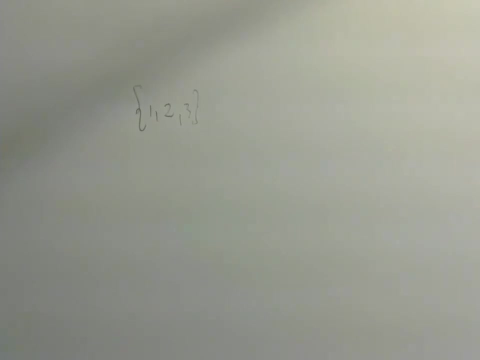 we're going to pretend to generate just one case, but we carefully follow how many choices we made while generating that one subset. So imagine that we have to make a decision. We're generating a subset. Are we going to put one into that or not? 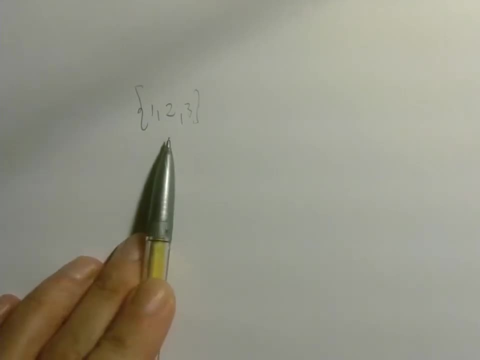 That's two cases, two possibilities. Then we have the same question to decide about: two: Are we going to select two into our subset? we're generating or not? And we have two choices with regards to three And therefore we're going to have: 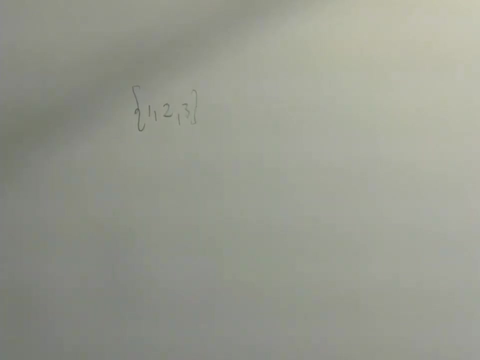 two times, two times two or eight such chain of decisions We can actually, for example, a yes, no, yes would create the subset one three: A no, no, no would create the empty set. A yes, yes, yes. 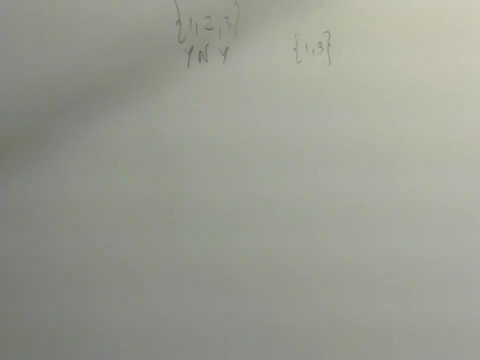 would create the entire set. We can also represent that using a tree diagram. We can say: the first question is: should we include one? Well, we can have a yes or a no. And now no matter what we did with number one. 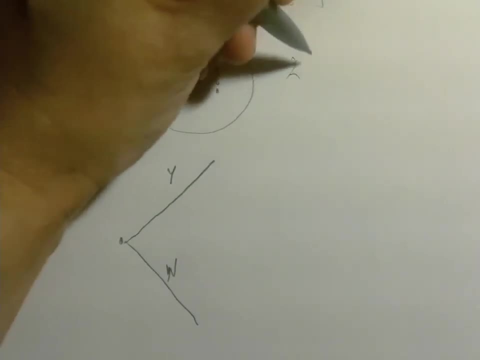 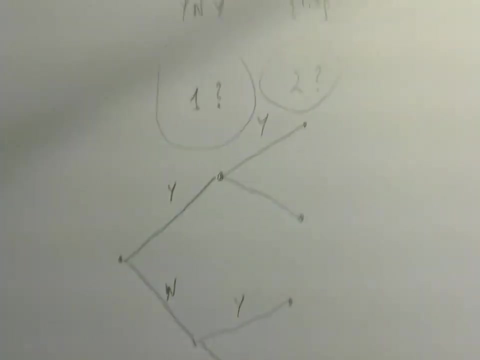 we can ask the following question: What about two? Do we want two into our subset? we're generating or not? And again there are two possibilities: Yes or no. And finally, we can ask the same thing about three. The problem with trees is they grow too big. 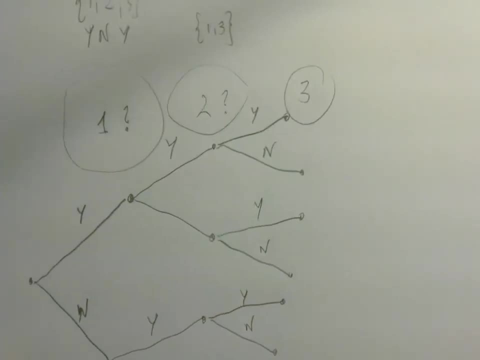 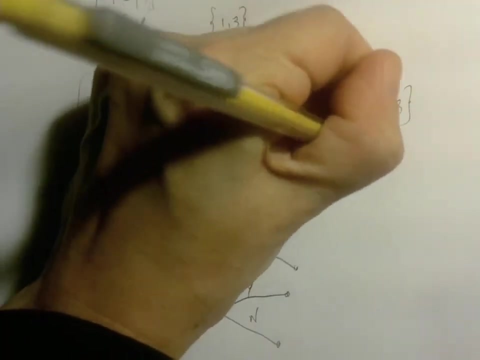 So we have two, four, six, eight little endings. Now, a yes, yes, yes, generated the set one, two, three. A yes, yes, no, generated one and two, Yes, no, yes would be one, three. 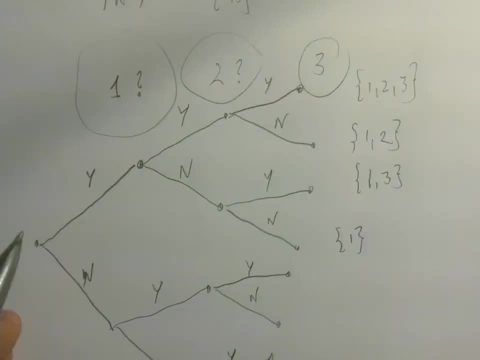 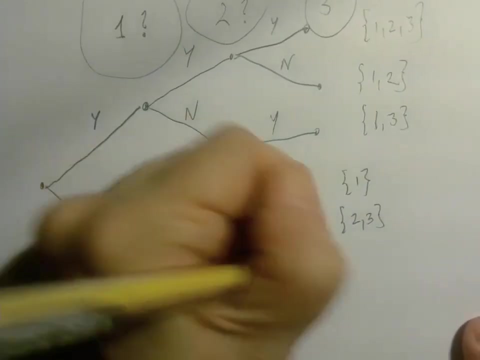 A yes, no, no would be just the one. No, yes, yes would generate two and three. We set no to one. only A no, yes, no would have the one element. set two in it. No, no, yes would be the one element. 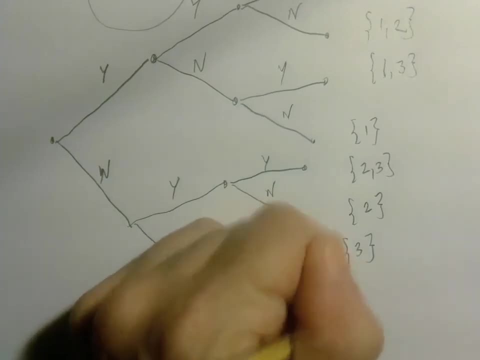 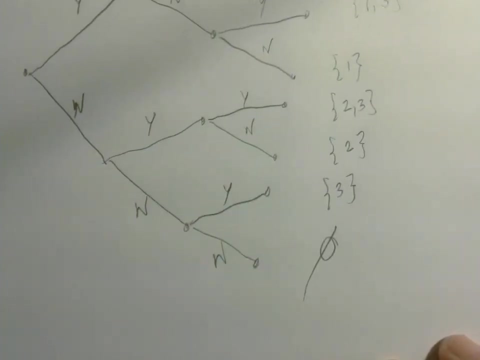 set three And no. no, no would be the empty set. So that is our one: two, three, four, five, six, seven, eight subsets. So this is now a combinatorial argument. So what are we left with? 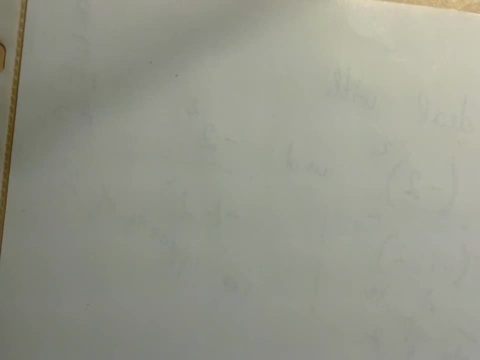 Now that we answered one question, we have the following questions: Is this outer symmetry universal? Will this stay with us? It looks like we have a very good argument And second, we have a ten element set. We now know that it has two to the tenth.